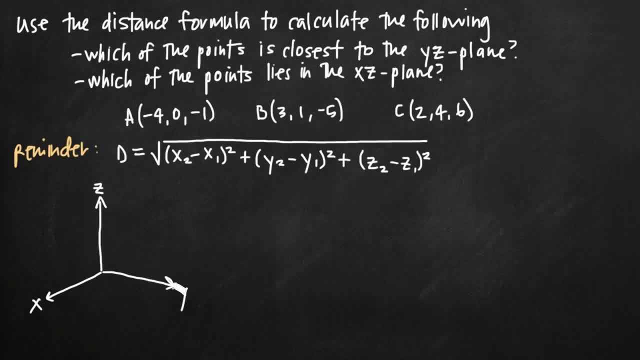 Well, the y z plane is the plane that includes the y and z coordinate axes. So the y z plane is the x z plane. So we can imagine it here. if we just draw a plane like this, It's going to be this plane that includes the y coordinate axis and the z coordinate axis. So this is. 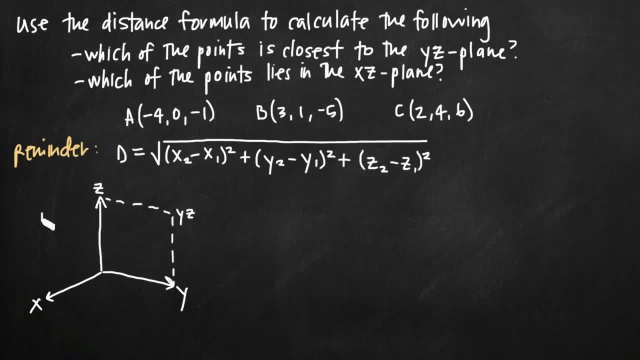 the y- z coordinate plane In the same way that the x- z coordinate plane would be the plane that includes the x and z coordinate axes. So this would be x- z. We can even draw our x- y plane here. It's sort of the floor of our coordinate system. So we're going. 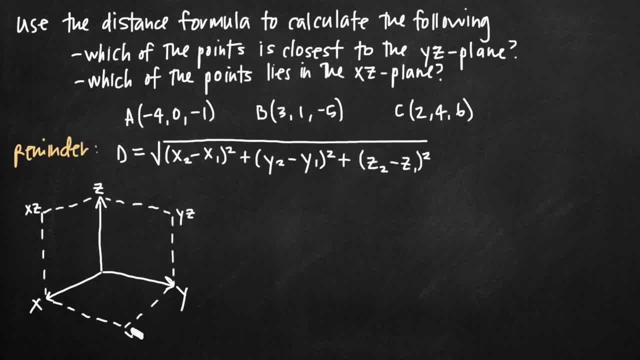 to draw a three-dimensional coordinate system, but it's right here, the x, y coordinate plane like this. So we have the three-coordinate planes of our three-dimensional coordinate system. Well, let's just take one of our points and figure out how we would calculate how. 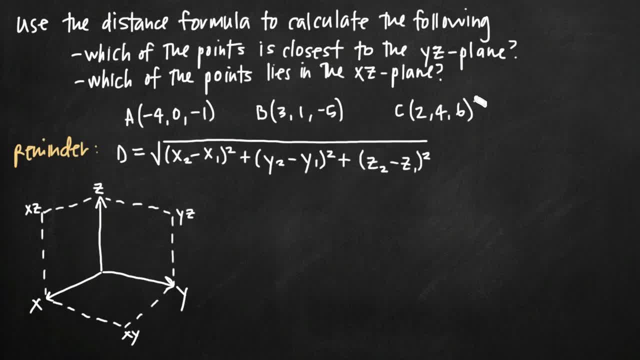 close it is to the y z coordinate plane. If we take, for example, probably the easiest point to do it with is point c, which is the coordinate point. So if we take that point and we graph it, let's say that we go out a distance of two on the x-axis. let's 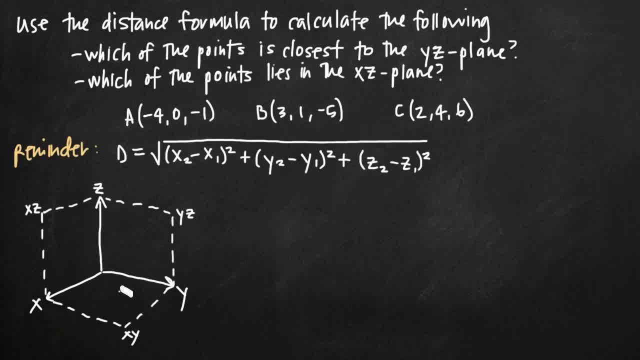 say that's about here, and then out a distance of four along the y-axis, so about double the distance, maybe here, And then we move up a distance of six up the z-axis here. so maybe that's about here, And we have this point. that's like floating in the middle of. 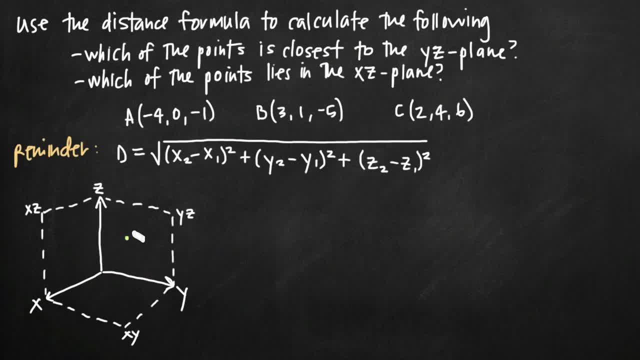 our space here. If we drew a box to represent where that was, we would say that the base of the box was about like this: two here out to four, something like this, and then up a distance of four. So we would say that the base of our box was about like this: two, four, six, like. 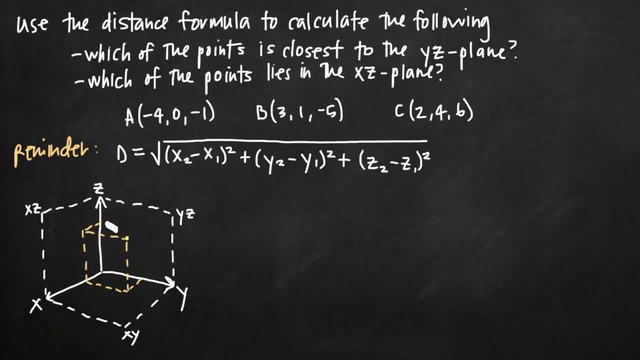 that And we could show that here from the origin that our box looked something like this out to this point, where that point- there, two, four, six- is the corner of our box. So there would be our box and there's our point, right there, floating in space at two. 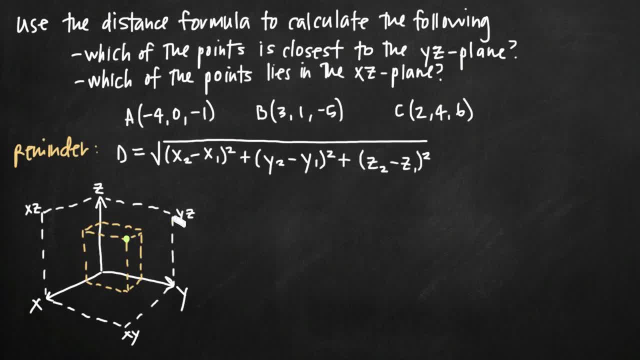 four, six. Now how do we figure out how close that is to the y z plane? Well, we want to draw a straight line directly from that point to the y z plane. Well, if we do that, we just move along this edge of the box here and we hit the y z plane at this point, right? 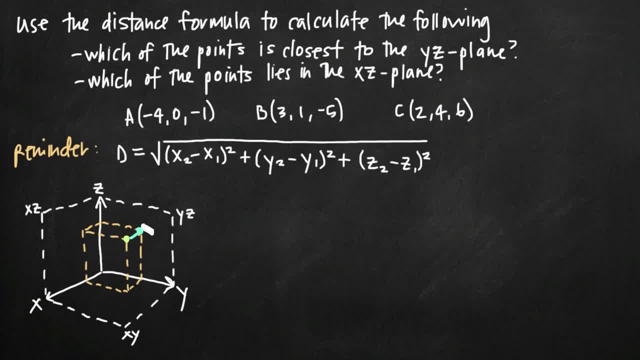 here. So we want to draw this straight line, getting directly to the y z plane. This is going to be the distance between these two points, or between this point c, here two, four, six and the y z plane. Well, all we've done here. what's the coordinate point here? 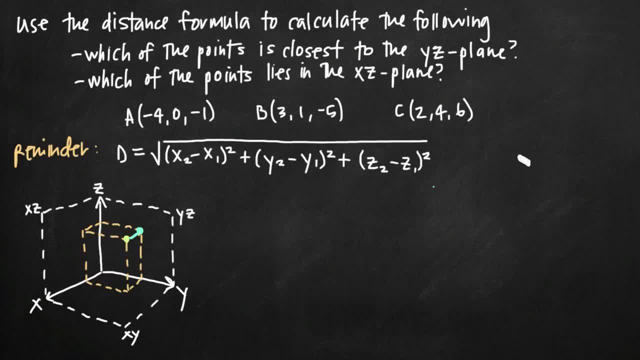 It's the y z plane. Well, we know that the y coordinate is still four. right, We're still out a distance of four on the y axis. We're still up a distance of six on the z axis. The only difference here is that the x coordinate of this new point in the y z plane is zero instead of. 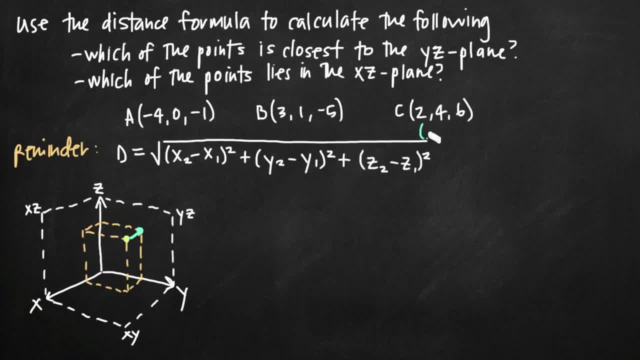 two. So this point here, the corresponding point, is just zero, four, six. Now what we learned from drawing this picture is that the point on the y z plane is going to be zero, four, six. Now what we learned from drawing this picture is that the point on 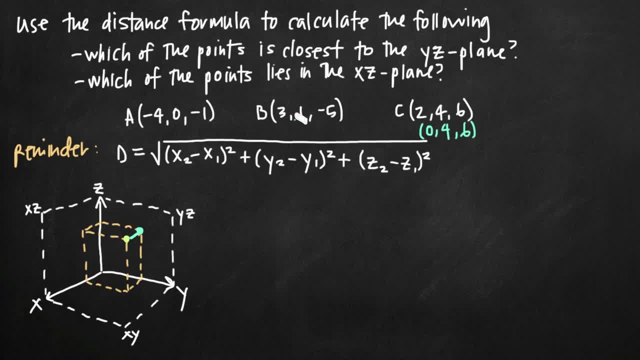 the y z plane that's closest to each of these points is the corresponding coordinate point, except that the x value in that coordinate point is zero instead of whatever it is in the original point. So the point on the y z plane closest to the point b would just: 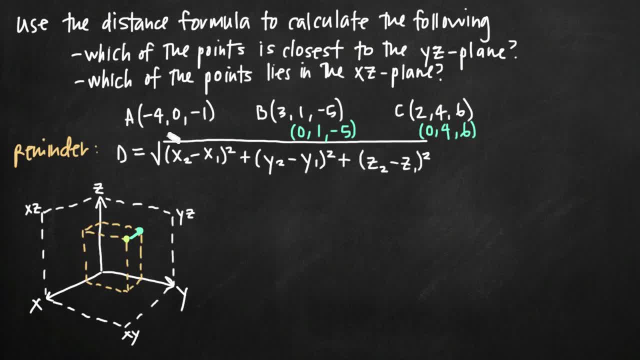 be zero. one negative five instead of three. one negative five. The closest point to point a that lies in the y z plane would be zero. zero negative one instead of negative four make it 0.. Now we have points between which we can calculate the distance using our distance. 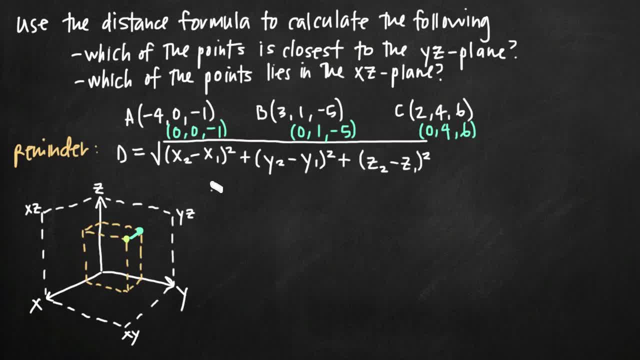 formula. So we're going to say that the distance between point A and its corresponding point on the y- z plane is going to be equal to the square root of x sub 2 minus x sub 1.. So we'll call all of our original points here, the x sub 1, y sub 1, and z sub 1, root. 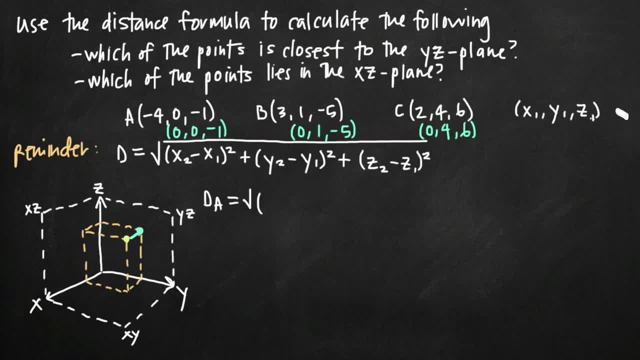 of x sub 1, and z sub 1 values. We'll call all of our secondary points here that we found our x sub 2, y sub 2, and z sub 2 values, So now we just have to plug them into our 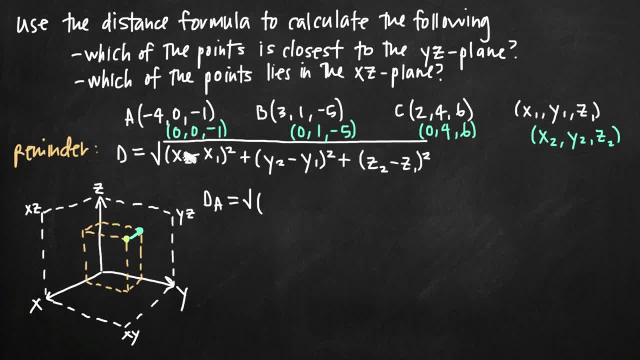 distance formula and we'll do one example and then move to our conclusion here. But we're looking for x sub 2, which we know here is 0 minus x sub 1, which is negative 4.. So 0 minus negative 4 and we're going to square it Y sub 2. we're grabbing here from our 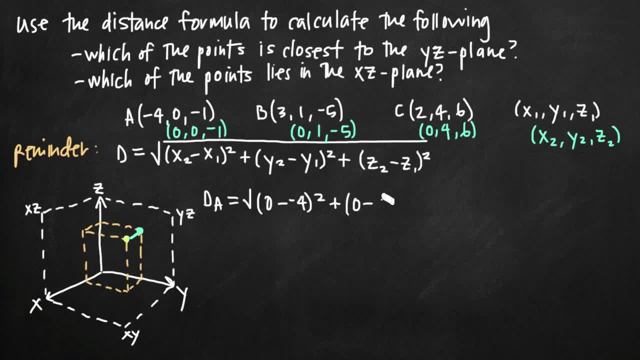 secondary point, which is going to be 0, minus y sub 1, which is 0, and we're going to square that. Then we're going to add to it z sub 2, which is negative 1, minus z sub 1, which is negative 1, and we're going to square that as well. So here is what emerges, Our y points. 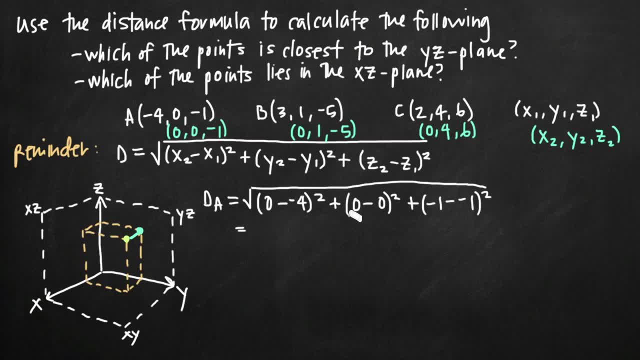 and our z points are always going to be the same. So 0 minus 0 is going to be 0.. Negative 1 minus a negative 1 is negative, 1 plus 1 or just 0. So negative 1 minus a negative. 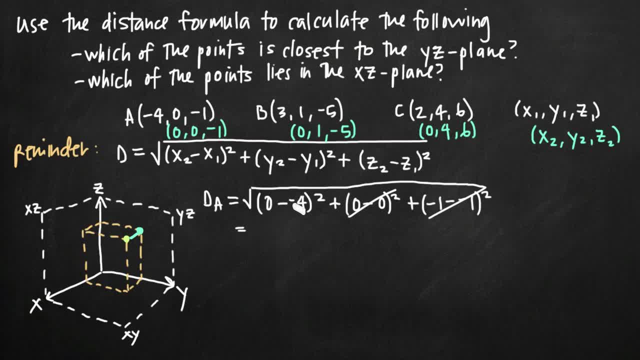 1 is 0. So that's going to go away. 0 minus a negative 4 is 0 plus 4.. So we have positive 4 squared, which is 16.. We're looking for the square root of 16. So we're going to get positive. 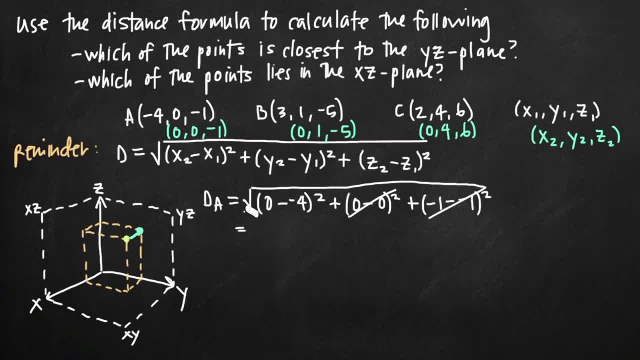 or negative 4, but we're talking about a distance here, a physical distance, So we don't include that negative value. We just say that the answer here is 4.. The distance between those two points is 4 units. What we should notice here as an emerging pattern is that if we 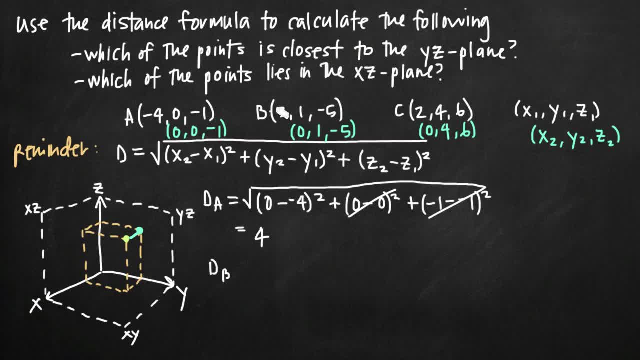 went and calculated the distance between the original point B and its corresponding point in the y z plane. what we're going to notice is, in the same way that we calculated the distance between point A and its corresponding point in the y z plane, the y and z coordinates. 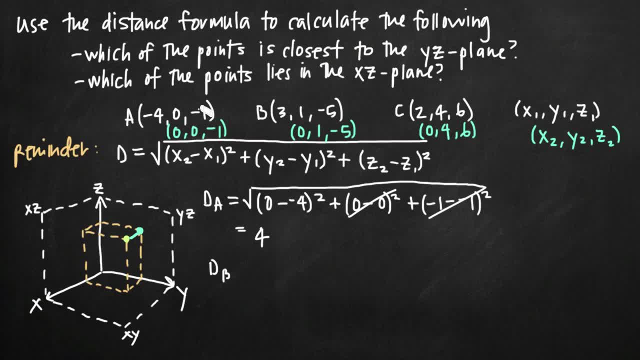 because they're the same, because we have here 0, 0 and negative, 1, negative 1, 1, 1 and negative, 5, negative, 5 and 4, 4 and 6, 6.. Those are always going to go away. We're. 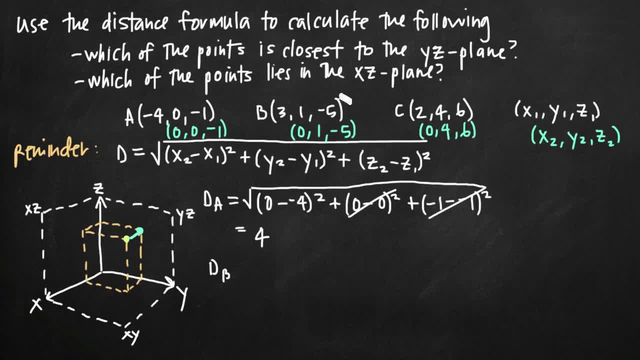 going to have 1 minus 1, negative 5 minus a negative 5.. They're always going to go away. They're all going to cancel. So really, all we need to do is calculate the distance between the x values. So we could simplify this to calculate the distance between B and its corresponding. 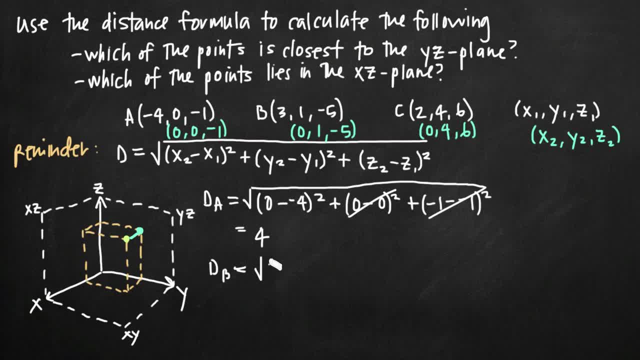 point on the y- z plane and just say: the square root of our x coordinate here 3, minus our second x coordinate, 0,. square it and be done with it, because the y and z coordinate points are going to cancel here And of course what we're left with is just 3 squared or the square. 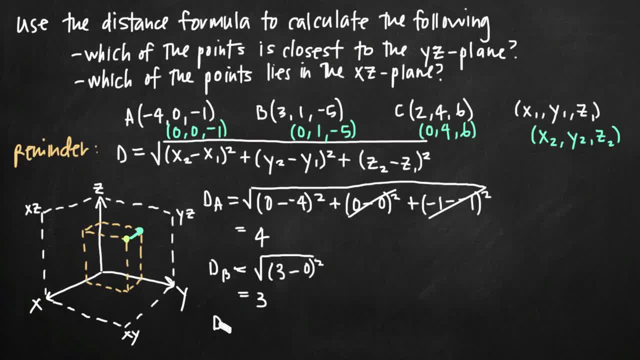 root of 9.. Which is going to give us 3.. Same thing here with d sub c. We're just going to do the square root of 2 minus 0, quantity, 2 minus 0, squared, and we're going to get 2 squared, which is: 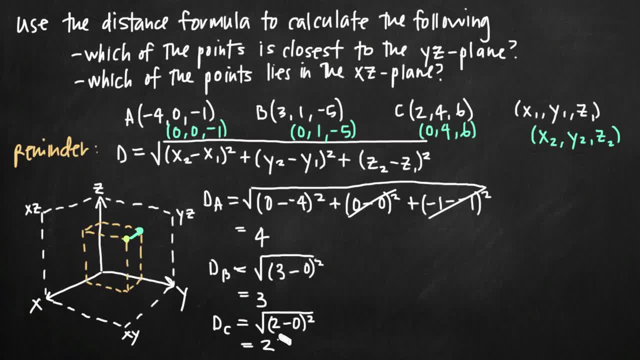 4.. Take the square root and we get 2.. What we see, then, is that these are the distances between points A, B and C and their corresponding points on the y z plane. Because d sub c is the smallest value, we have 2,, 3 and 4 here. 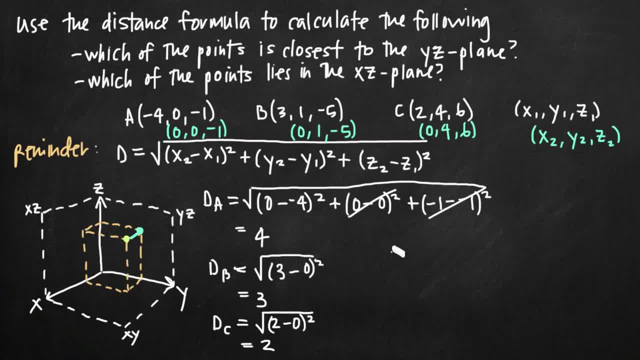 d sub c is the smallest value. We can say that the point C is the point closest to the y z plane. So that's how we figure that one out. Now this one's a lot easier. Which of the points lies in the x z plane? Well, of course, our x z plane is this plane, right? 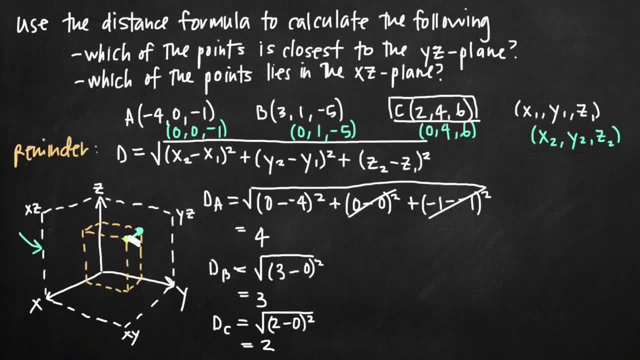 here this x z plane that we drew before. Which of the points lies in that plane? Well, what we can identify here is, for example, these points here In our box that we drew for point C, But these four points all lie in the x z plane, The 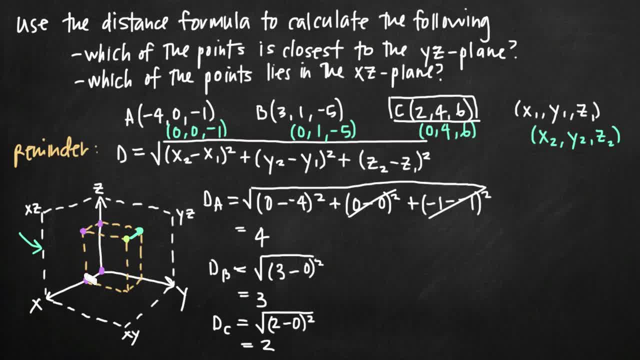 reason they lie in the x z plane is because their y value, the y value of each of these coordinate points, is 0.. Right, When the y value is 0, we're going to have a value that lies a coordinate point that lies in this x z plane. So we're just looking for one. 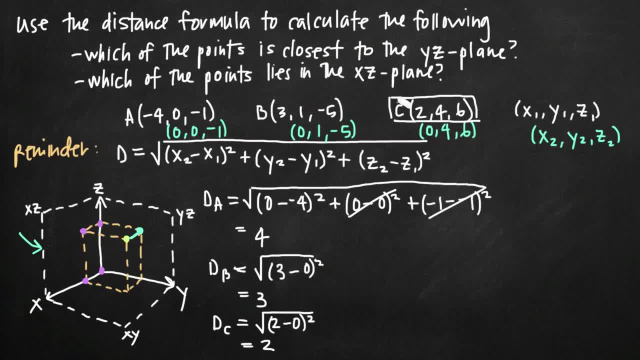 of our points that has a y value of 0 and we're going to have a coordinate point that has a y value of 0. And of course we can see that that's point A here, where the value or the coordinate point is. If we drew that here, we could go out a distance.